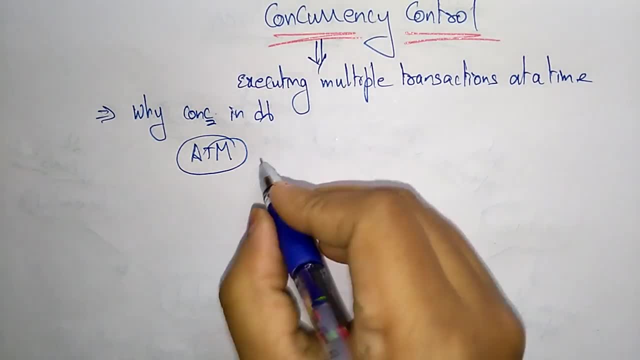 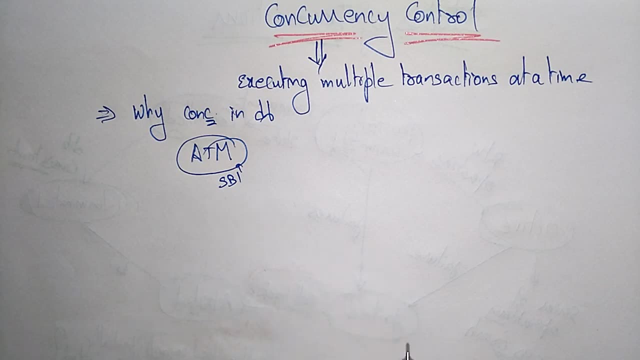 suppose, Okay. so if you take a ATM machine that is SBI bank, related to SBI bank, Suppose one person is withdrawing money in one of the ATM bank, Okay. if you are not withdrawing money in one of the ATM bank, Okay. if you are not withdrawing money in one of the ATM bank, Okay. if you are not. 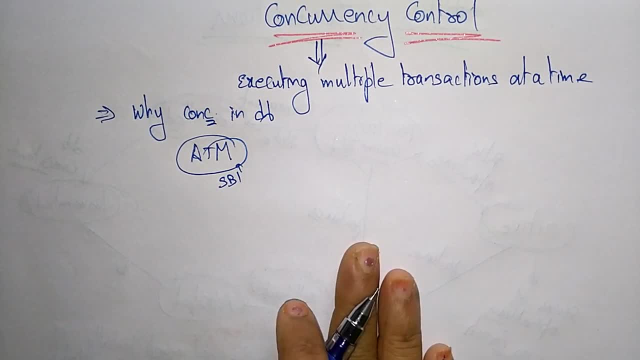 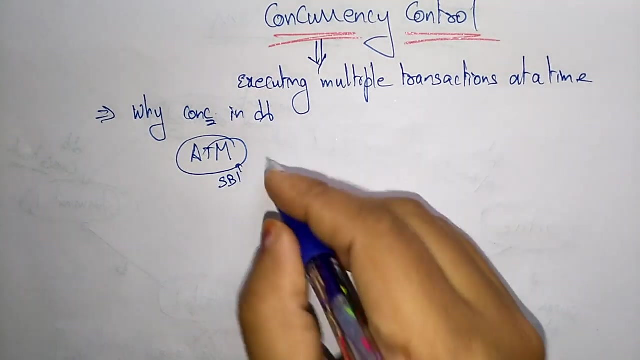 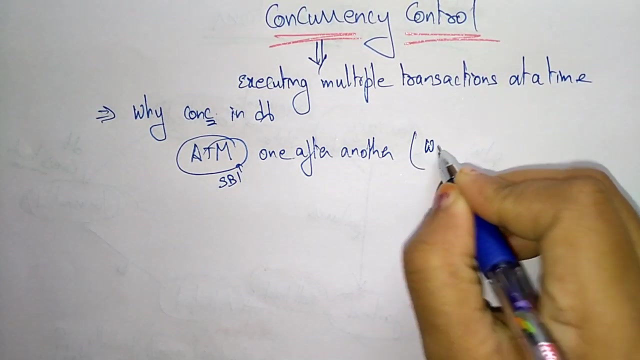 using the concurrency. If you are not using the concurrency, So the person, if he is using the ATM by withdrawing the money after the completion of his work, only another person can withdraw the money in another ATM. Okay means one after the another, One after another. So if we without concurrency, Okay. 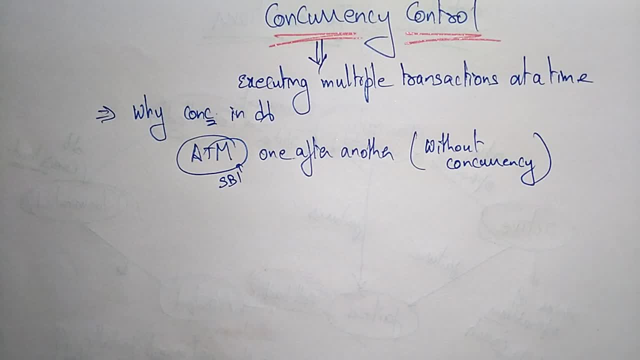 Okay. so then wastage of time is more because so many people are accessing the ATMs of the same bank at the same time in different places. If they wait that much of time, it is wastage of time will be more. So for that reasons, we are going for the concurrency. Okay. you can take another examples for railway reservations: Okay, in the railway reservations also, if you are accessing the TATKAL tickets. Okay, if you are accessing the TATKAL tickets. Okay, if you are accessing the TATKAL tickets. Okay if 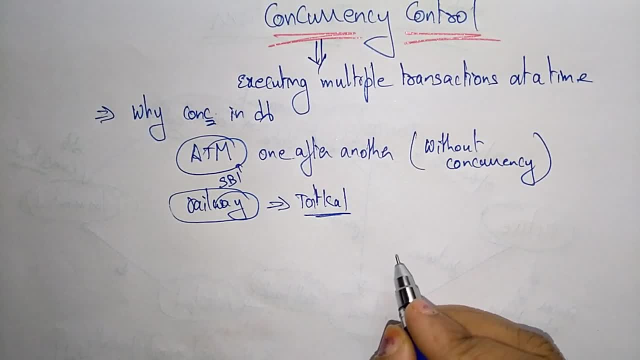 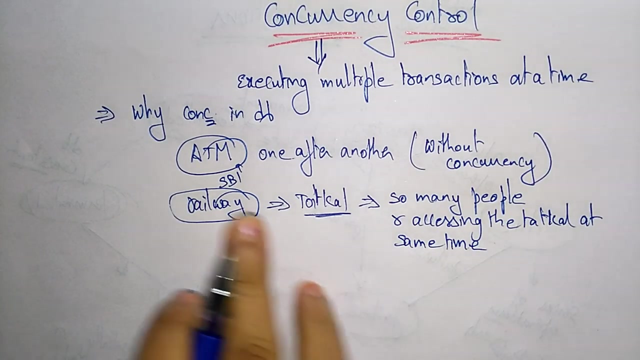 If you are accessing the TATKAL tickets at that particular time, so many people are accessing at a time, So many people are accessing the TATKAL at same time, So in that case also the concurrency is important because it is executing multiple transactions. 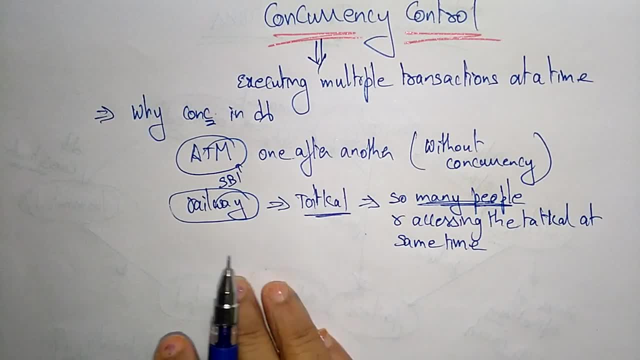 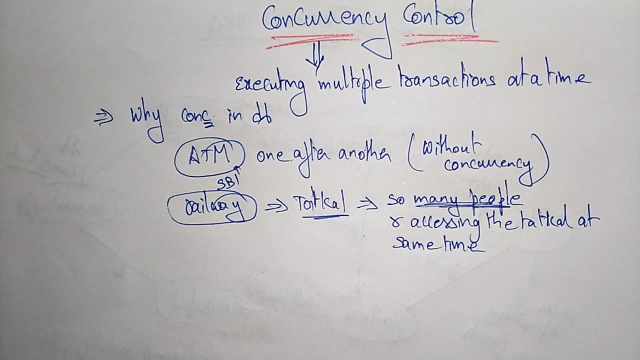 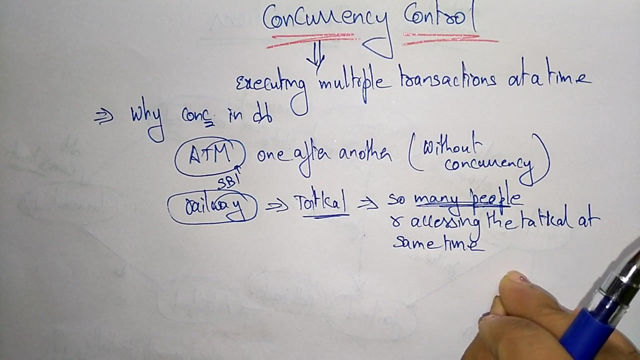 Different people are executing at the same time, accessing the same portal at the same time. So here one thing is: whatever the transaction is doing by single person, they thought that those transaction will be in isolation. Means whatever the transaction he is doing, the person that thinks I am the only person who accessing this railway reservation. 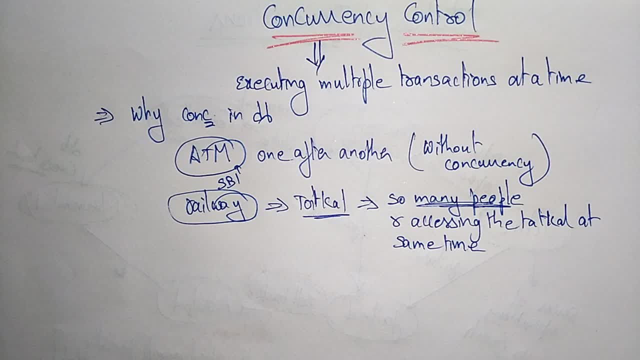 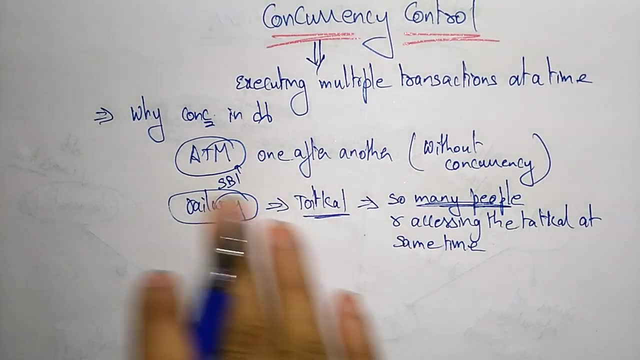 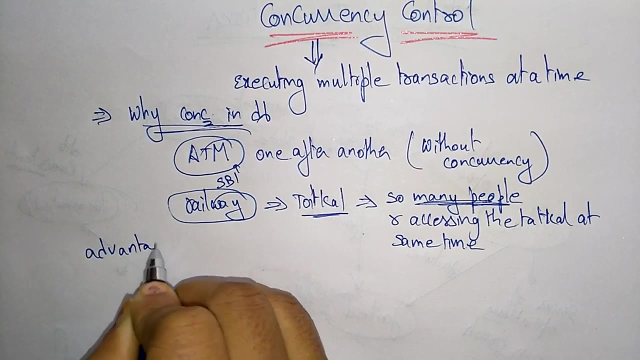 Because he is having that much of features like he can Access. he can, he can book the ticket. OK, so this is why we are using the concurrency in database. What are the advantages of using these concurrency in database advantages? OK, so the advantage is the waiting time. 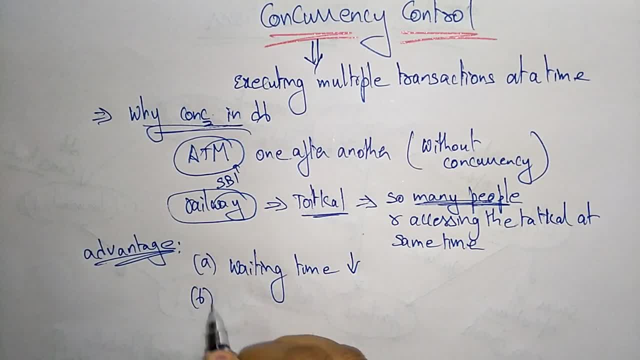 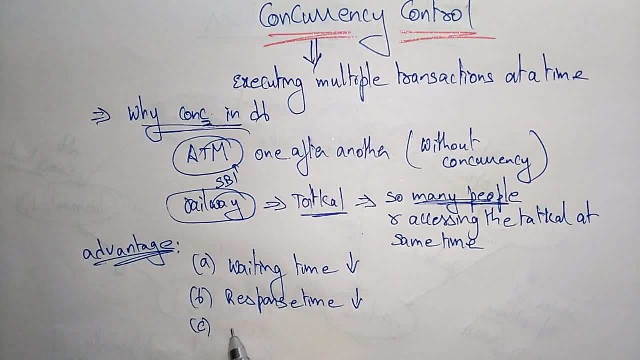 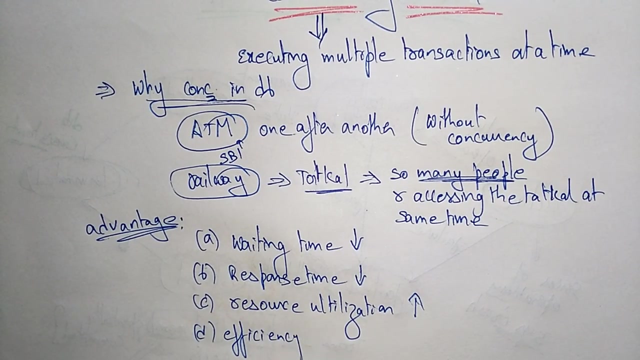 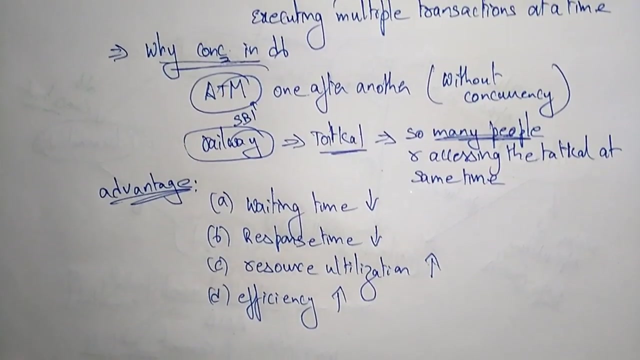 Will be decreased. Response time Will decrease. Resource utilization, so so many people can utilize the same resource, so resource utilization may increase. Efficiency will be increased. the system performance and efficiency will increase. so these are the advantages of using concurrency. So, even though these many of advantages will be there- why we are controlling the concurrency- 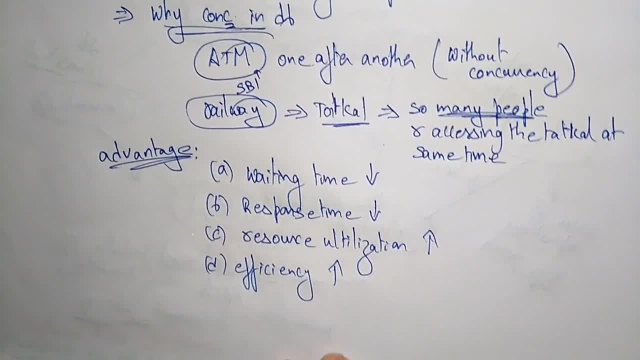 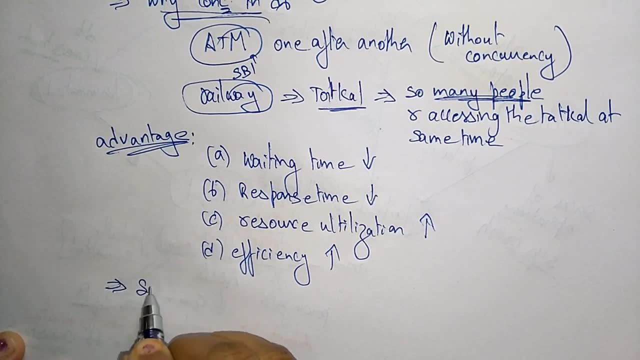 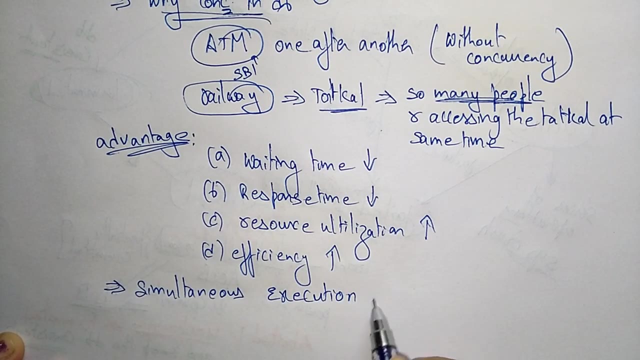 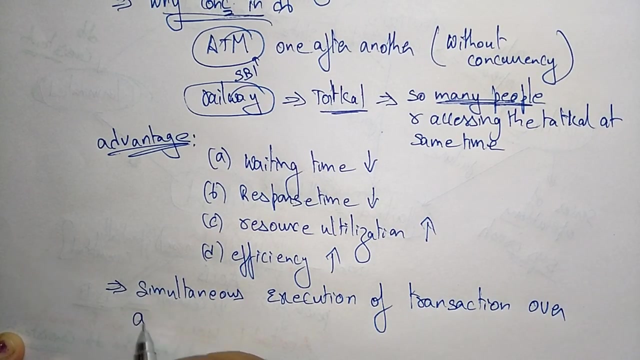 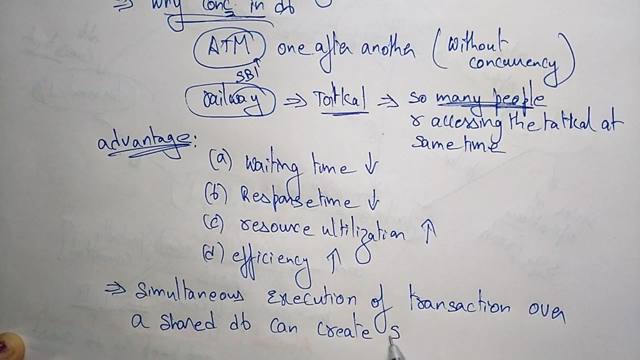 OK, So what is the problem that is raising in using the concurrency control? So here you have to be. note that simultaneously, The simultaneous execution of transactions Over a shared database Can create A, A, A, A, A, A. 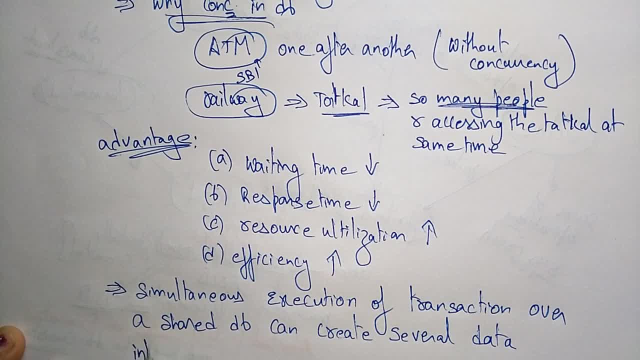 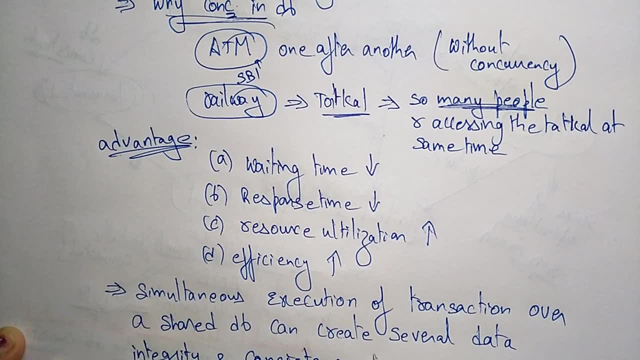 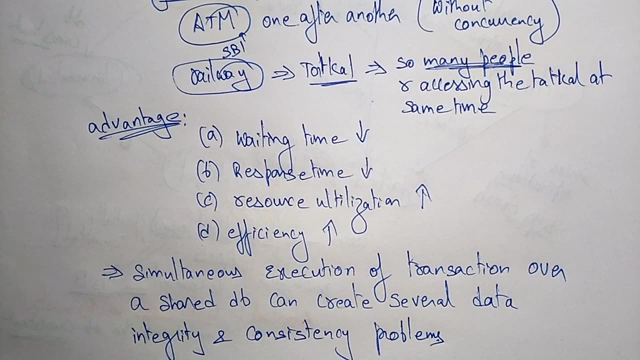 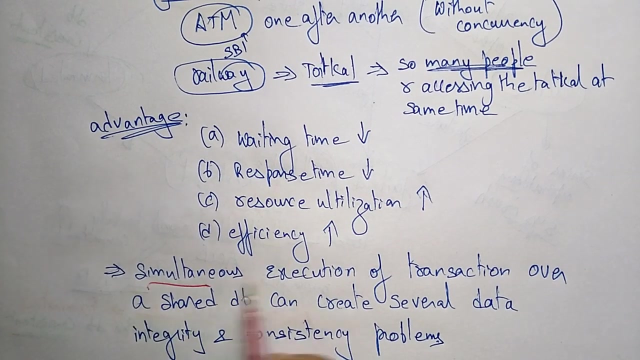 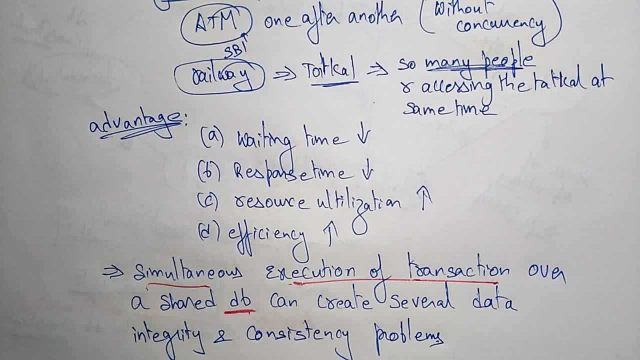 over a shared database. A single database is there. Suppose the database is SBI database. Simultaneous execution- So many people are withdrawing the money at the same time in the shared database- can create several data integrity and consistency problems will be there. 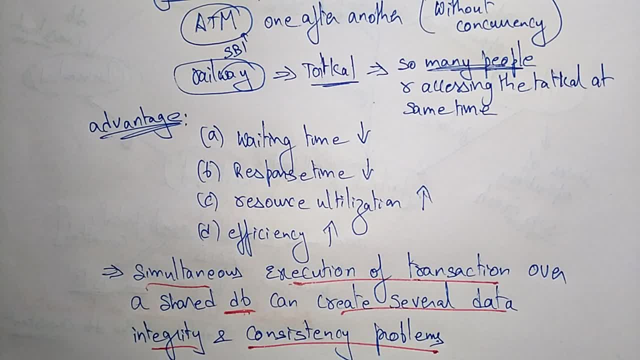 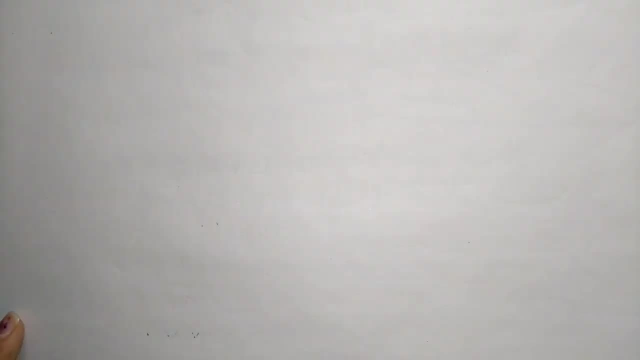 So what are those problems? Even though it is executing fasting, the response time is decreased, resource utilization is more. even though those many of advantages Here, some integrity and consistency problems will be there by using the concurrency. So the main problems of using this are So the main problems there are three main problems will be there. 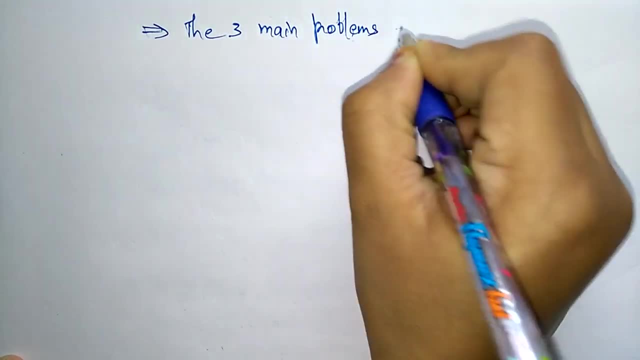 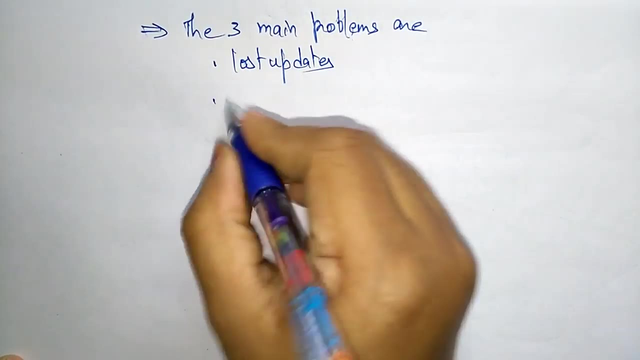 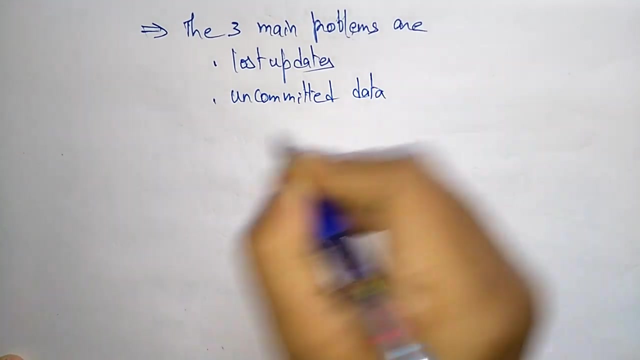 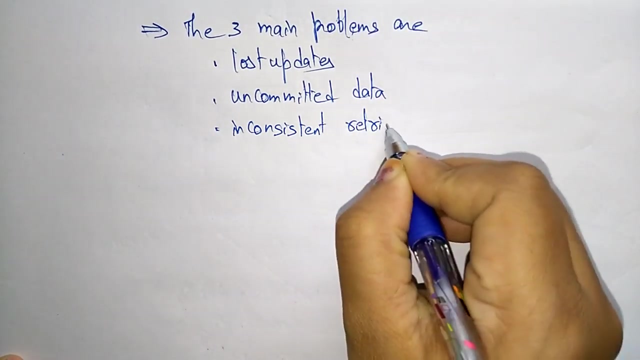 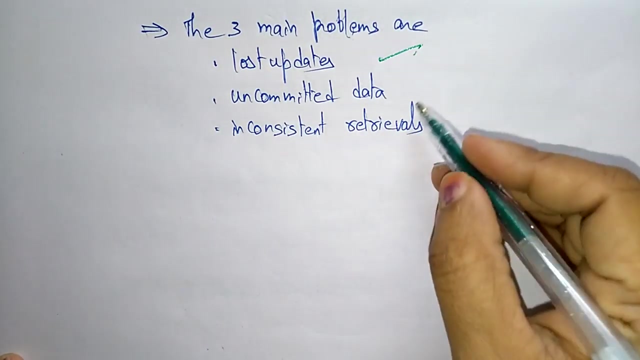 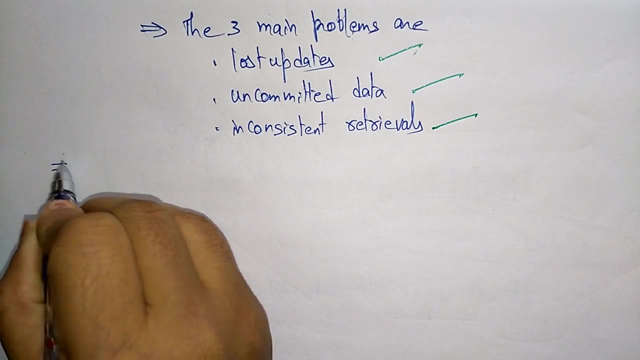 The three main problems are: The first one is lost updates. Swallow Updates will be lost. Uncommitted data, Uncommitted data, Inconsistent retrievals. Okay, So these are the three problems that are facing the concurrency Control: Lost updates, Uncommitted data, Inconsistent retrievals. So let us see the conflicts that are arised in the serializability of a transaction. 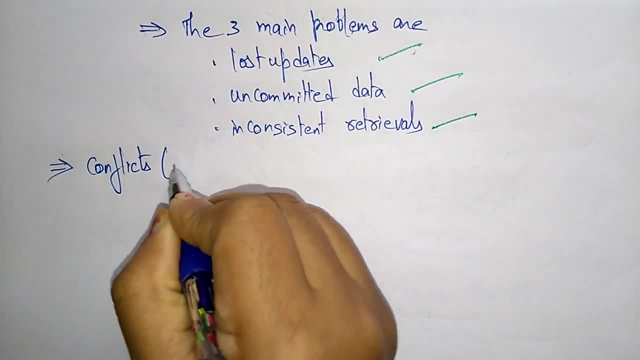 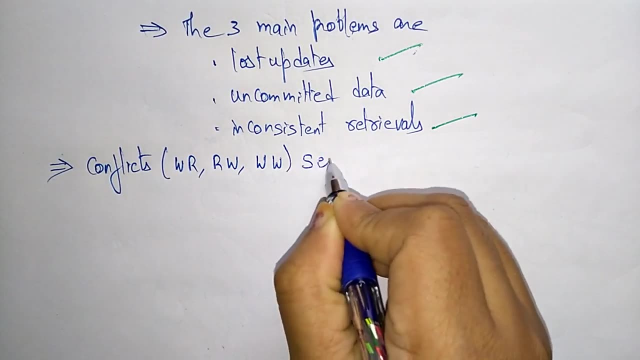 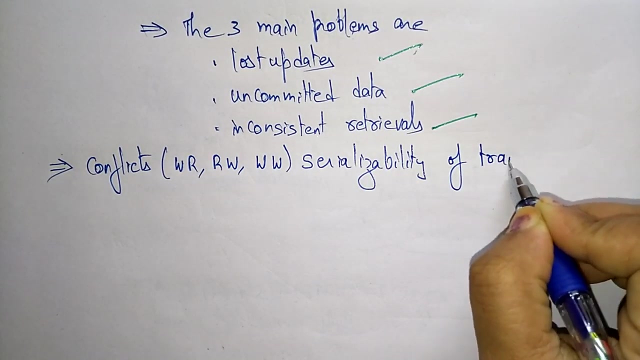 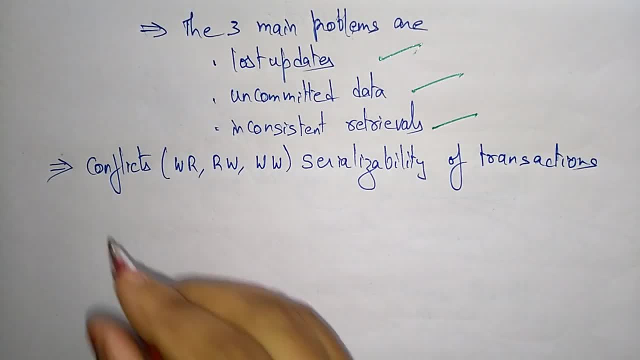 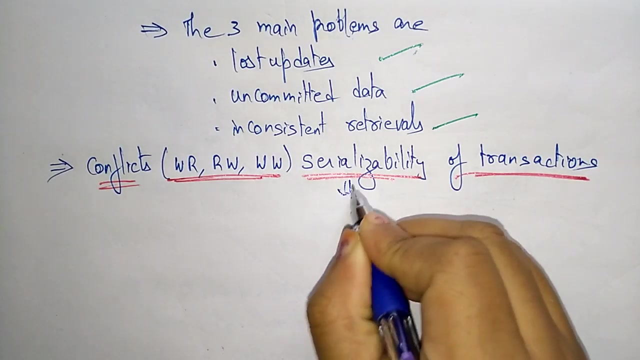 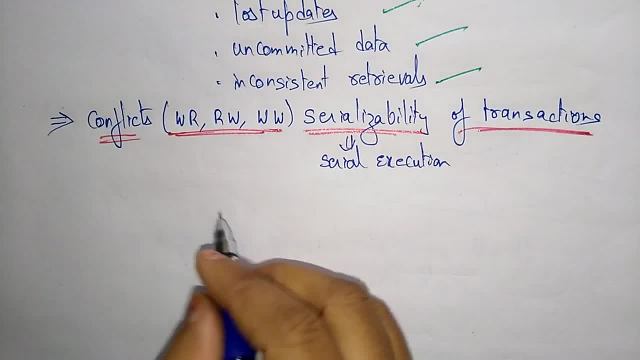 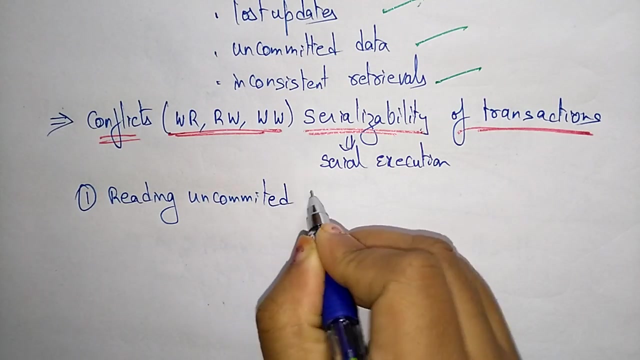 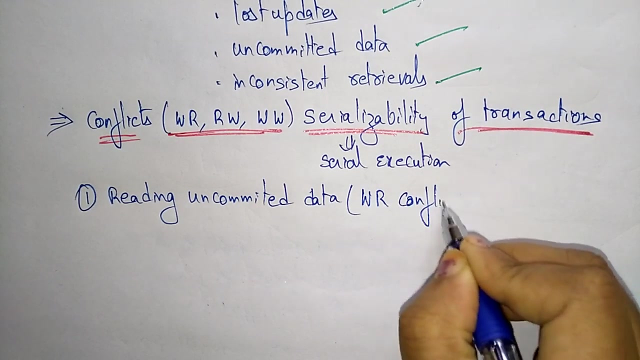 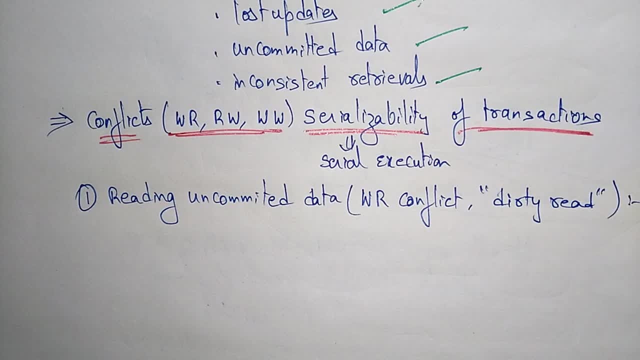 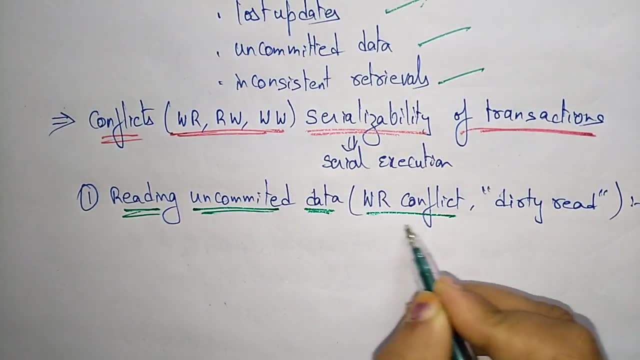 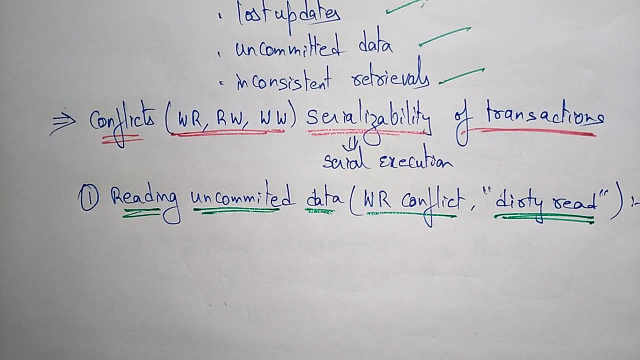 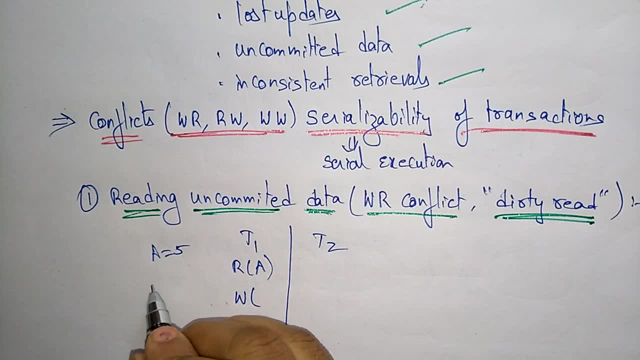 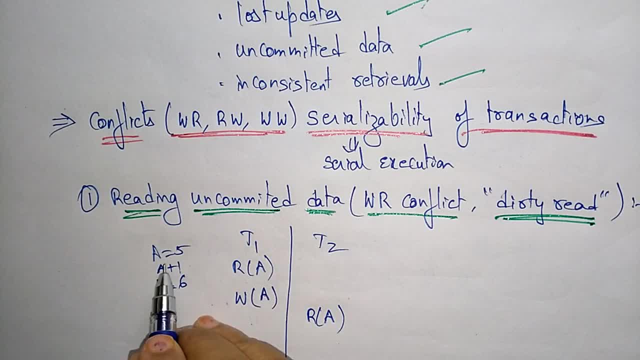 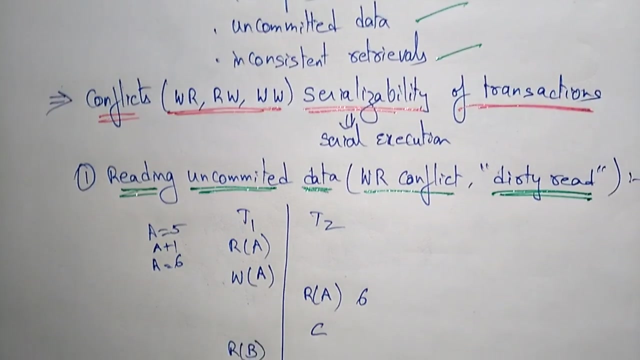 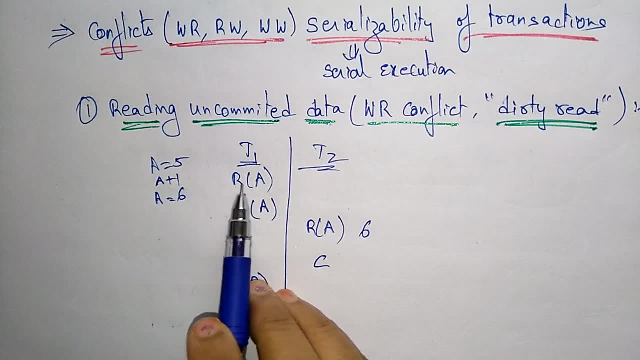 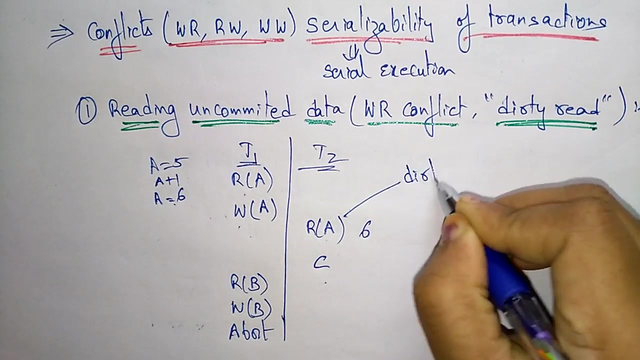 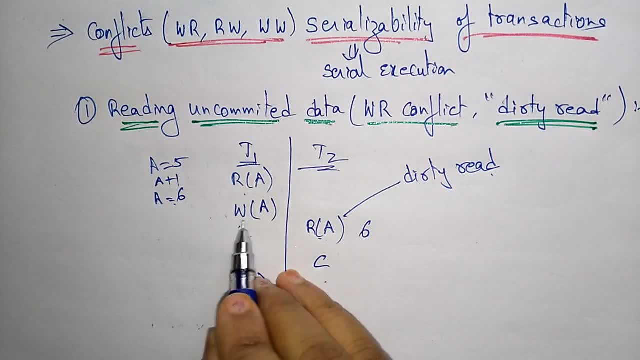 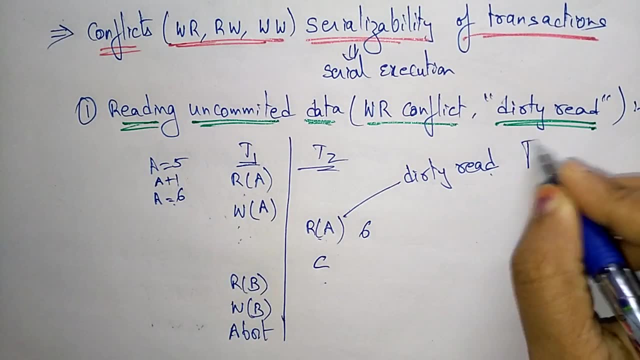 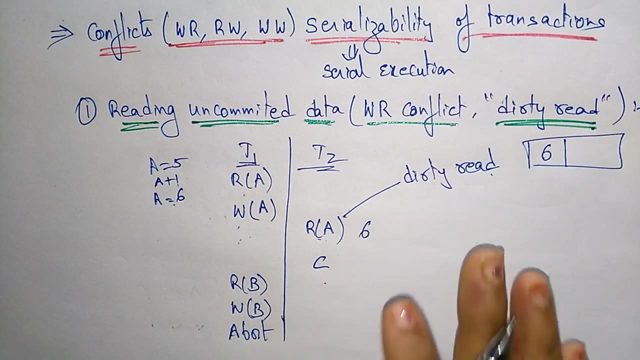 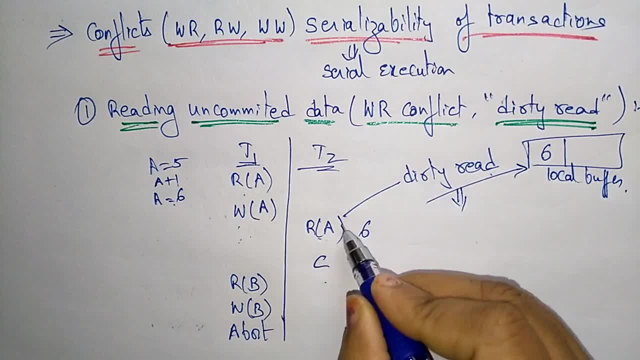 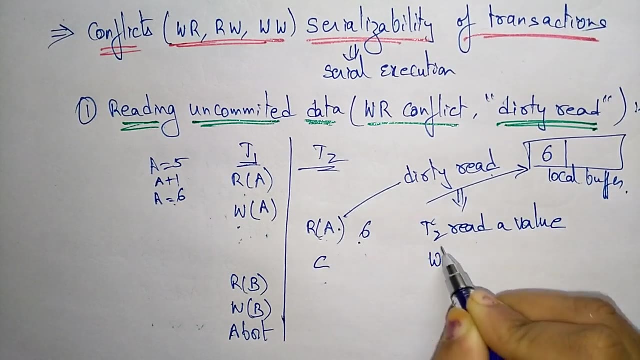 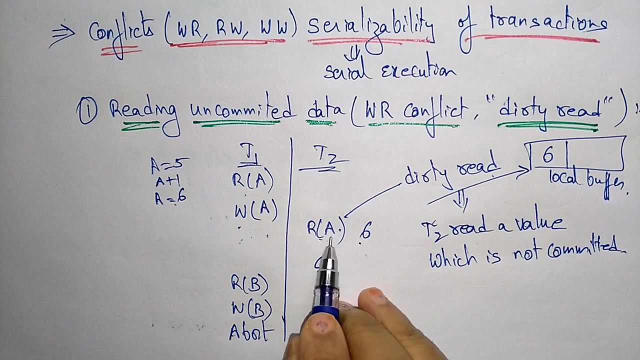 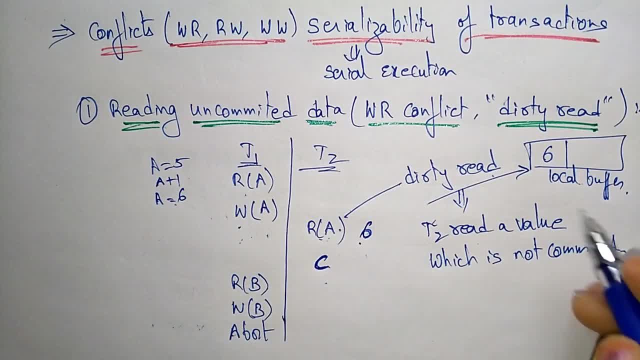 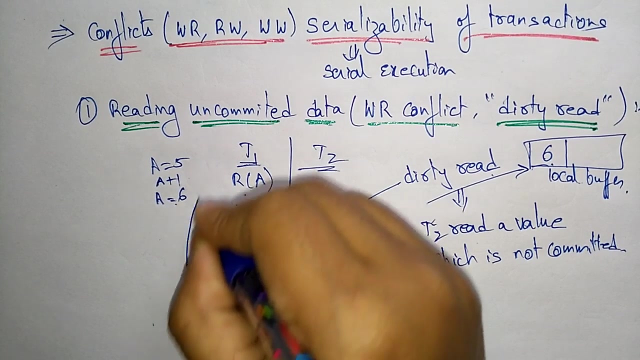 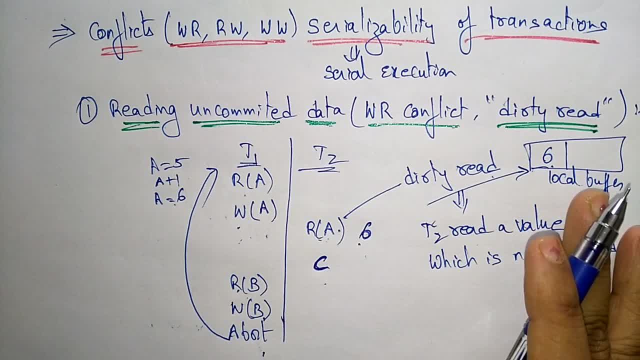 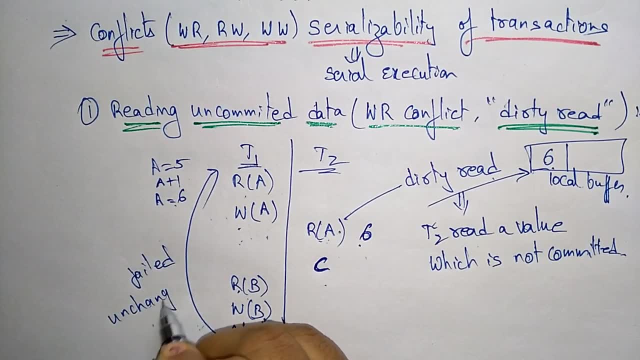 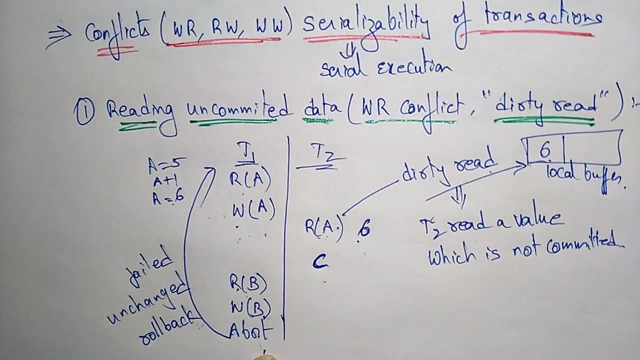 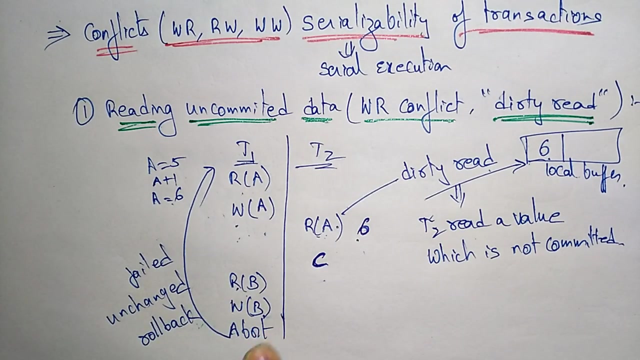 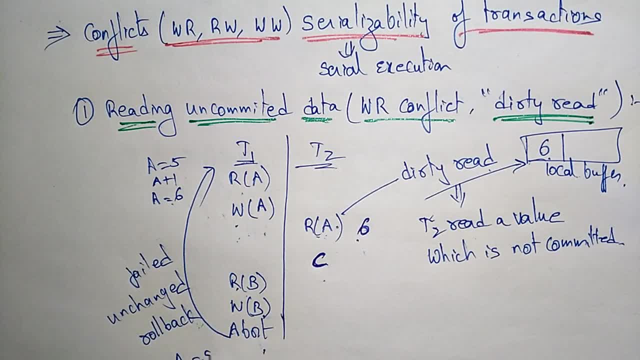 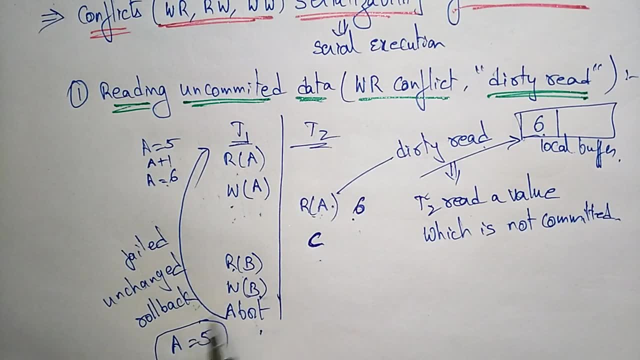 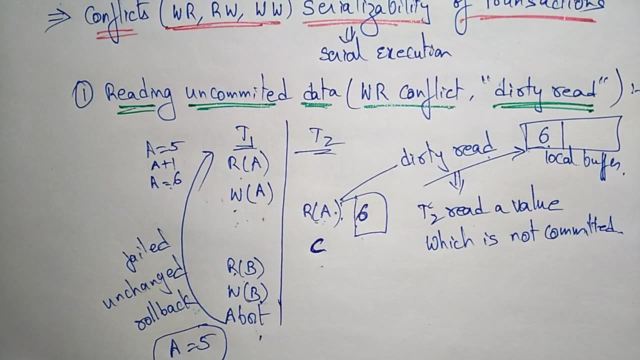 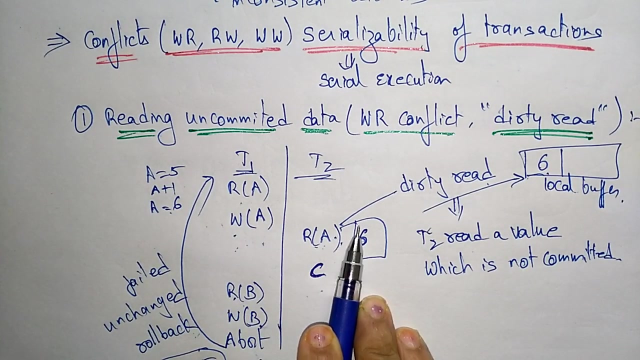 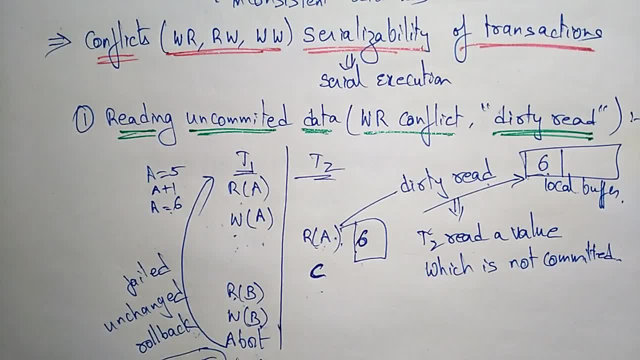 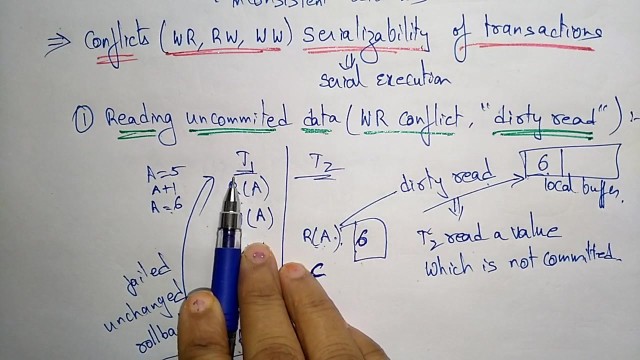 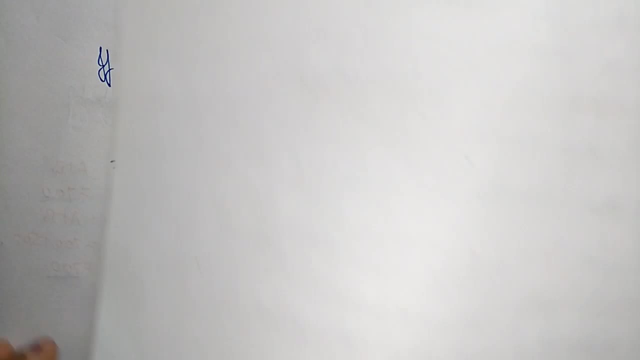 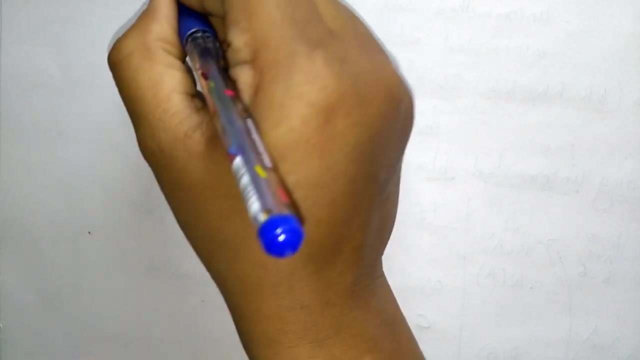 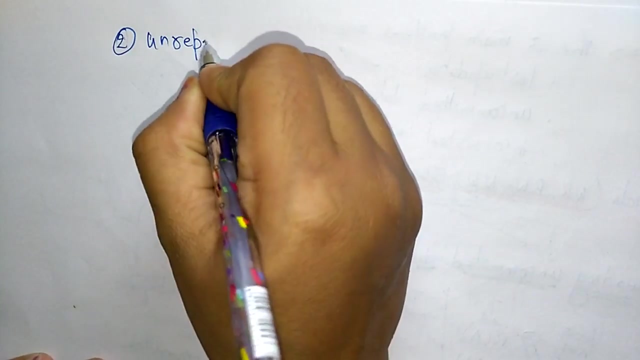 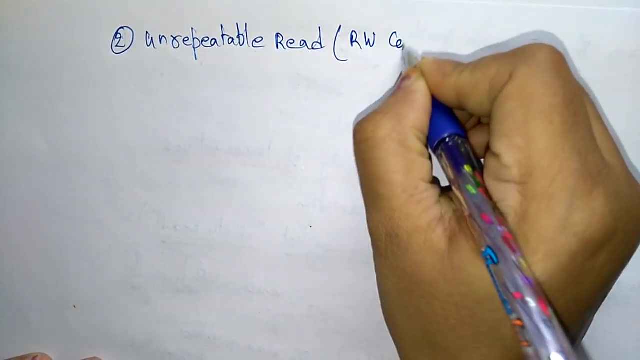 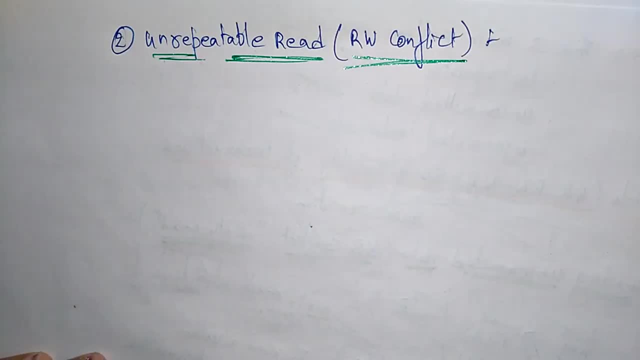 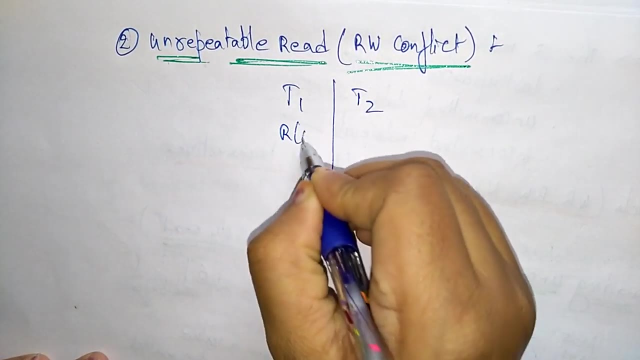 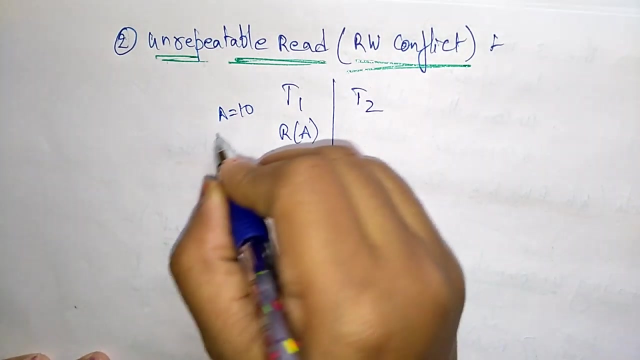 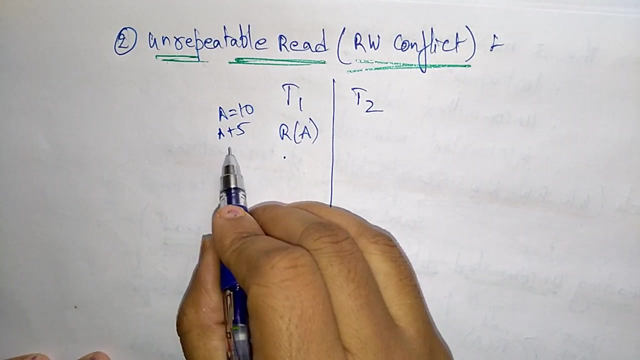 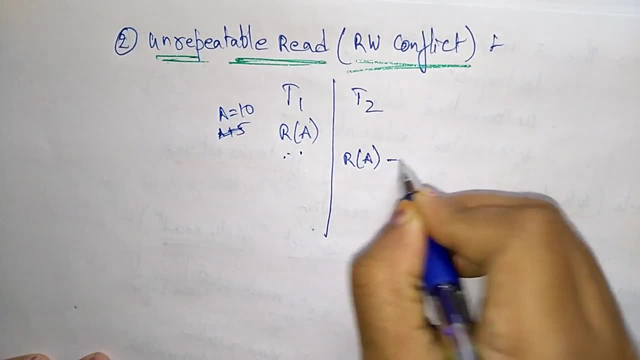 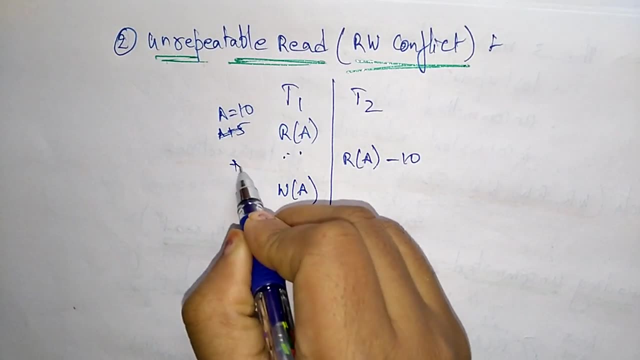 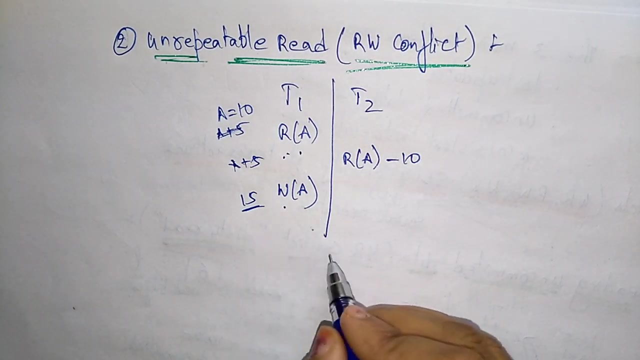 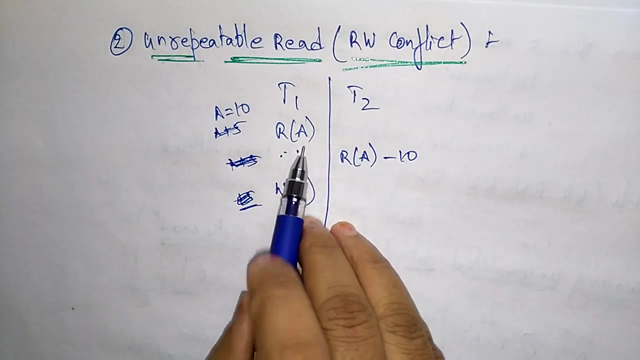 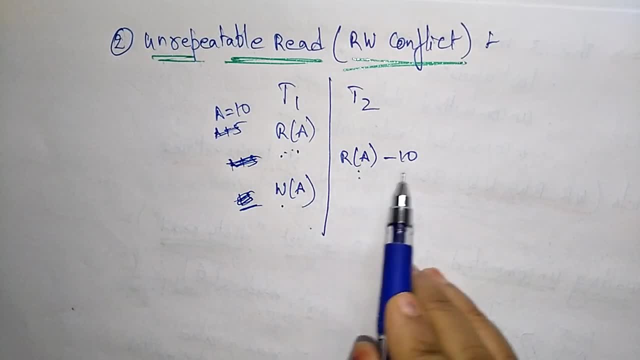 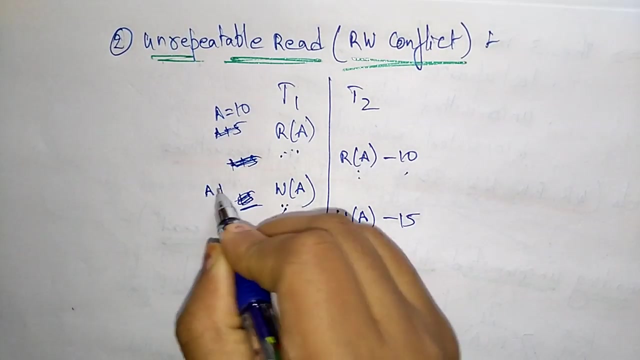 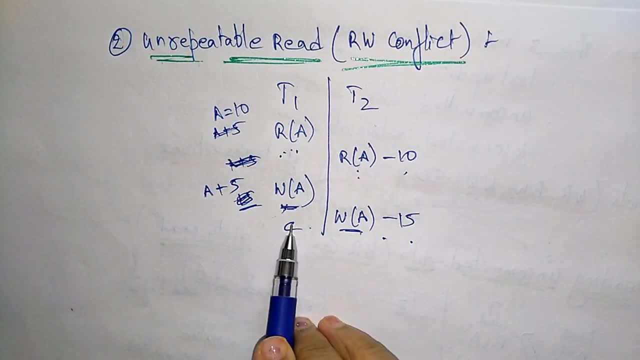 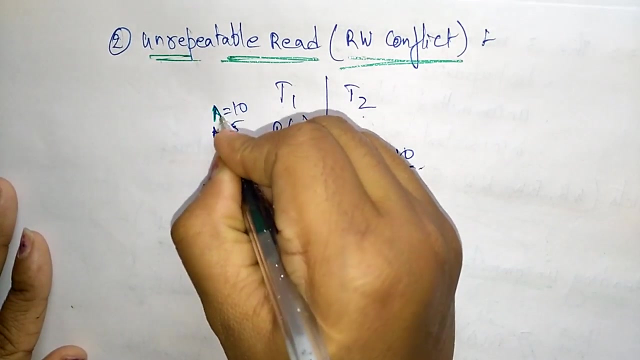 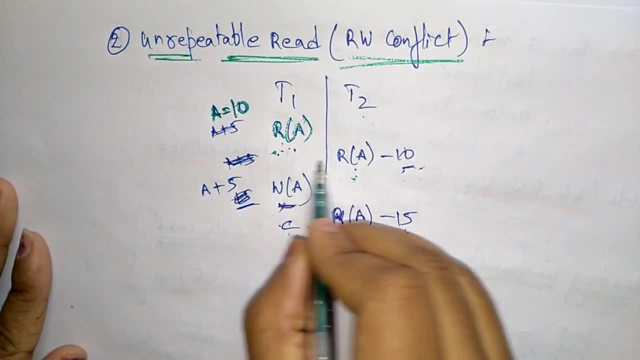 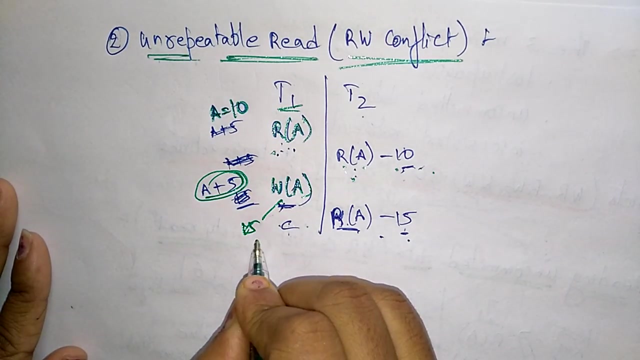 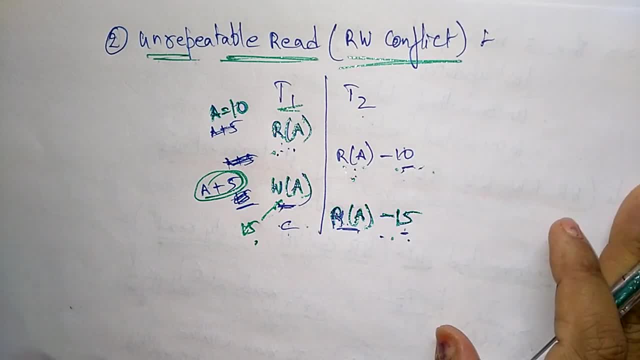 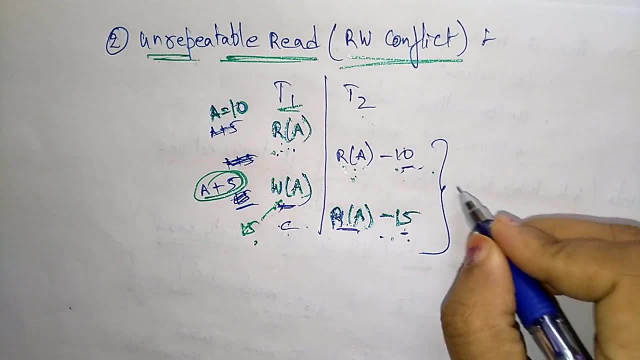 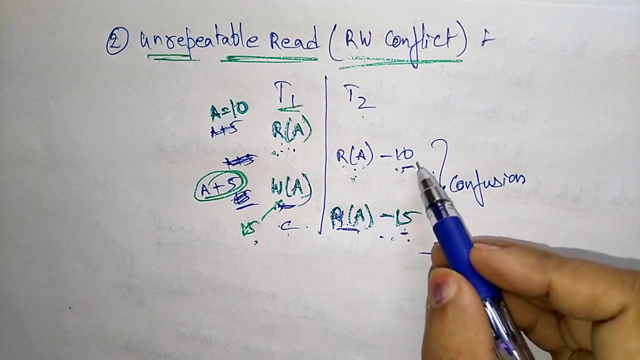 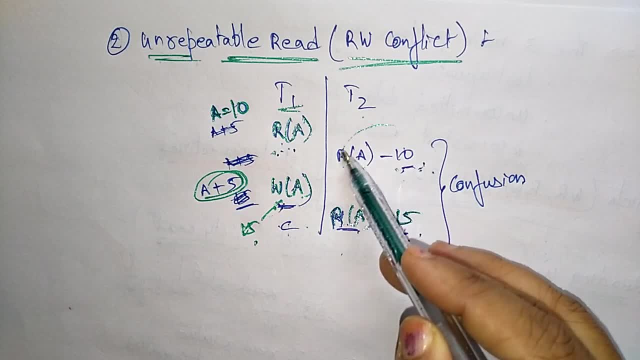 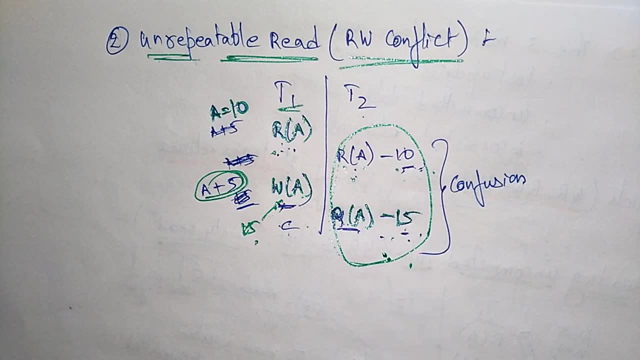 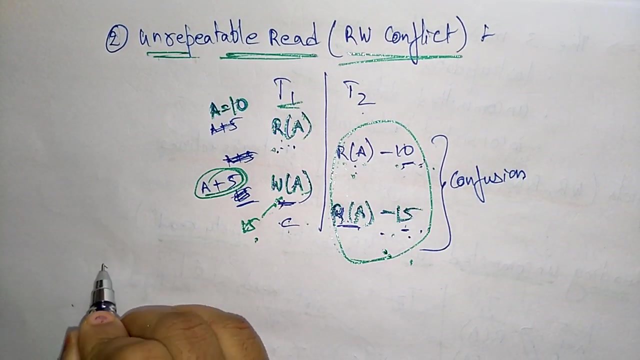 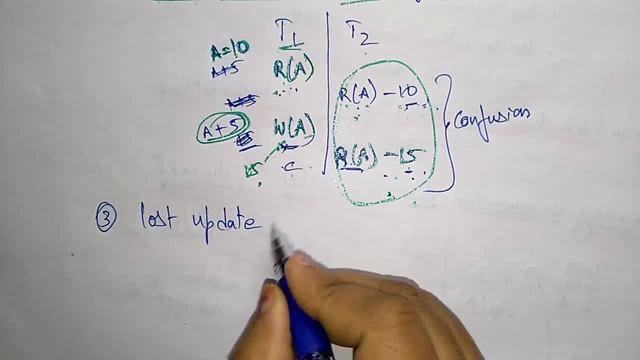 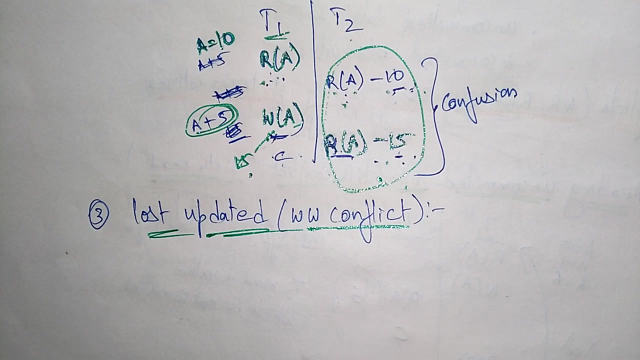 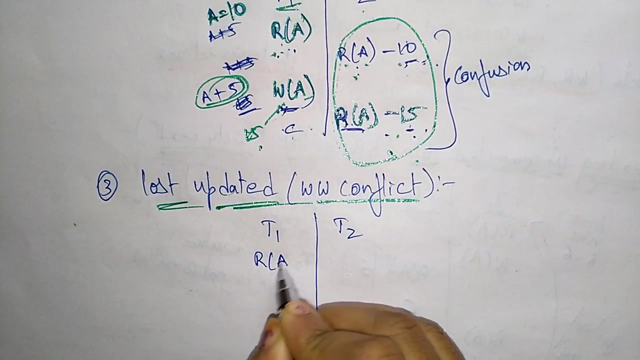 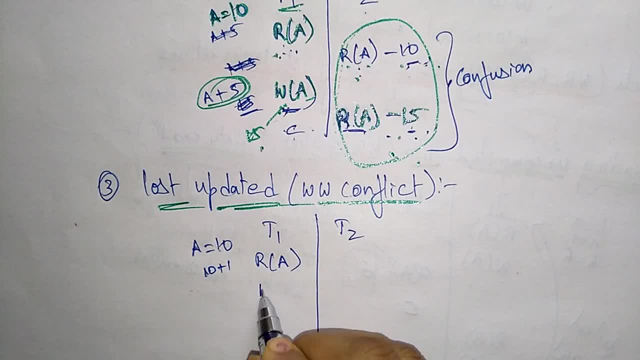 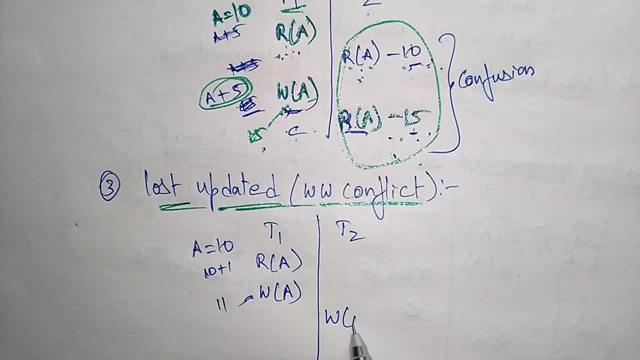 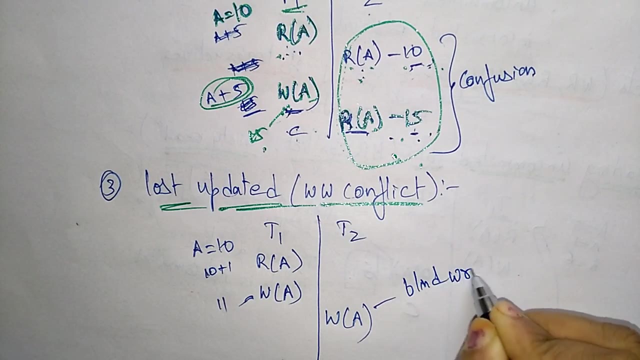